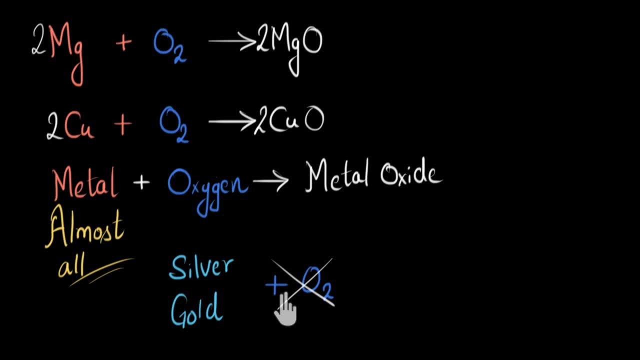 they are not going to combine with oxygen, We will not get oxides of silver and gold being formed, And that's why we say almost all metals combine with oxygen to form metal oxides. So with this let's try to rank our metals. 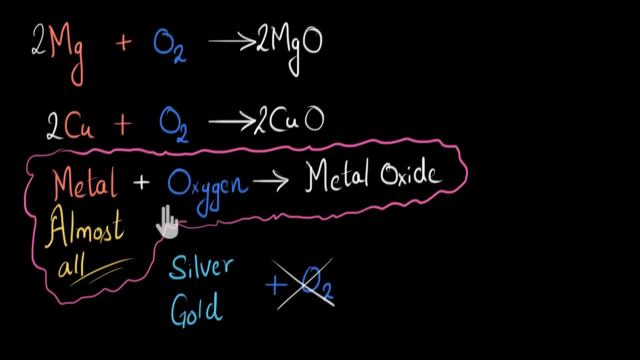 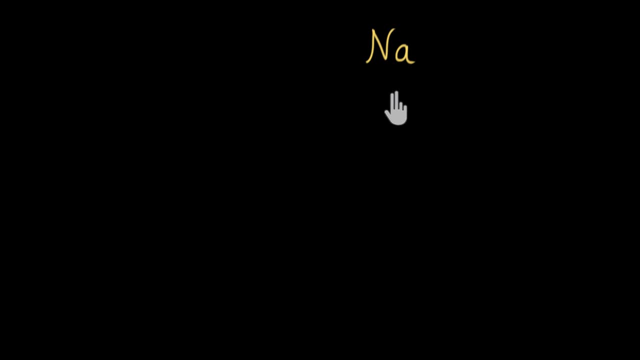 according to how vigorously or how weakly they react with oxygen. So first let's begin with sodium. If you heat sodium in open air, it will catch fire and start burning very vigorously. We will have a vigorous reaction. In fact, this can even become explosive in nature. 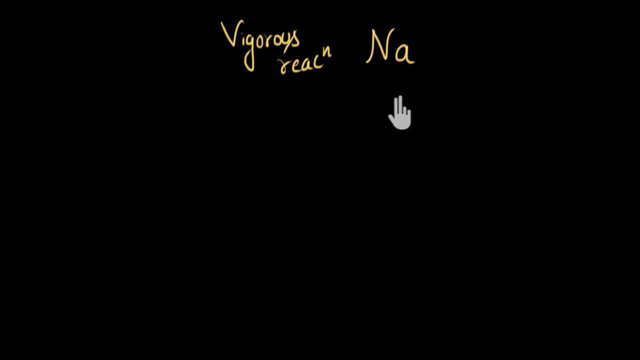 So be very careful while carrying out this reaction. In fact, we don't even need to heat it, Just keep it out in the open air, and it might react automatically with oxygen and catch fire. That's why we never keep sodium in the open. 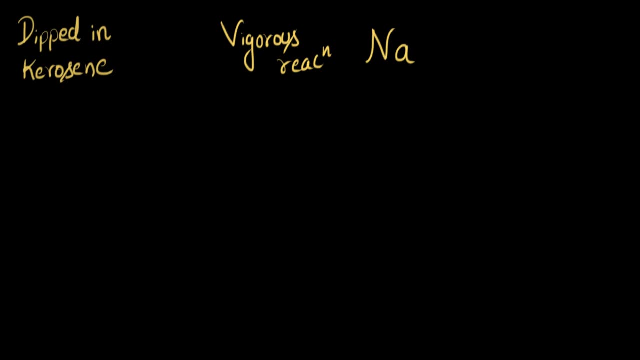 We store it by dipping inside sodium. We store it by dipping inside kerosene, So it never comes in contact with air or water. And just like sodium, potassium is also very reactive. Its reaction with oxygen is also very vigorous in nature. 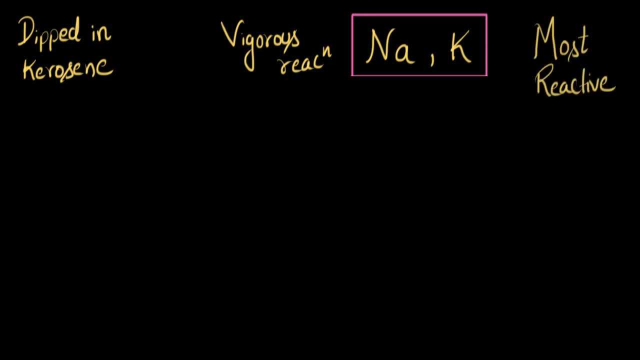 So these are the two top most reactive metals that we have. Next we have magnesium. We have already seen that when we burn magnesium it catches fire and it burns with a dazzling white light, So it is also very reactive, But in comparison to sodium and potassium, 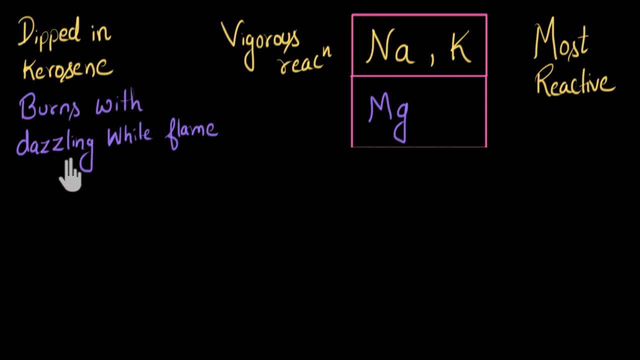 it can only come second. It's no match for them Now. next up, I have metals such as aluminum, zinc, iron and copper. Now, all of them react in a similar fashion with oxygen to form their oxides, And that's why I have grouped them together in a single box. 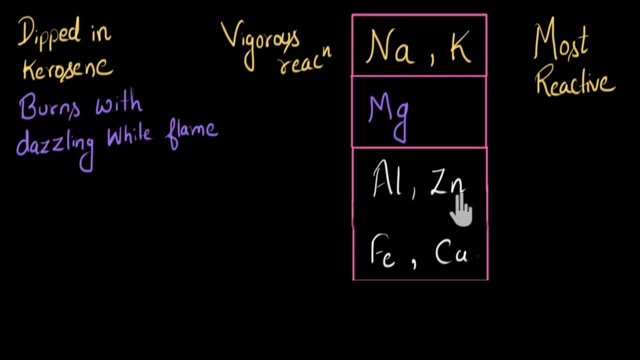 It's pretty hard to actually tell which one among them is more reactive. So let's see which one is more reactive. Let's see which one is more reactive And their reaction is not as vigorous as sodium or magnesium, And that's why I've put them at a third rank. 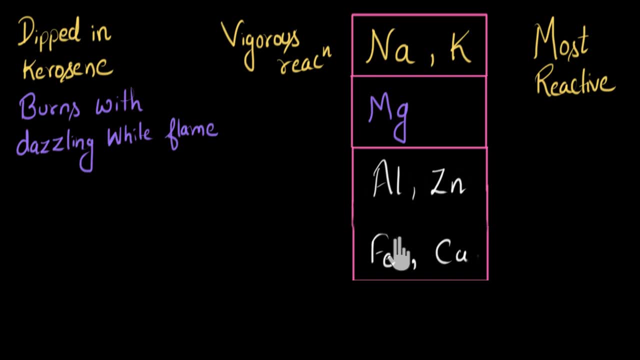 Now, even among them aluminum, zinc and iron, they will burn and react with oxygen to form their oxides, Whereas copper it does not burn. It will get hot and then it'll react with oxygen to form copper oxide, whose color is. 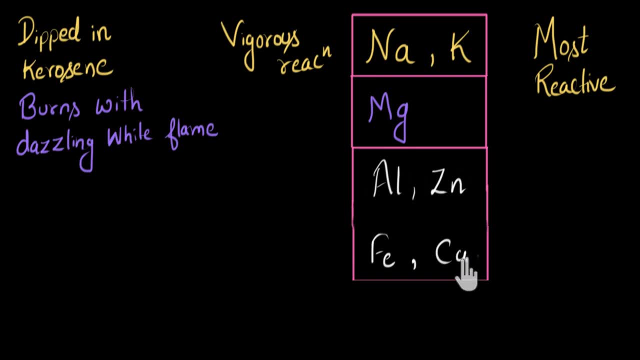 black, And that's why you'll see a color change From copper color to black color. Okay, with this, I have listed out few of the metals that will react with oxygen to form oxides. Now, after this, we have metals such as gold and silver. 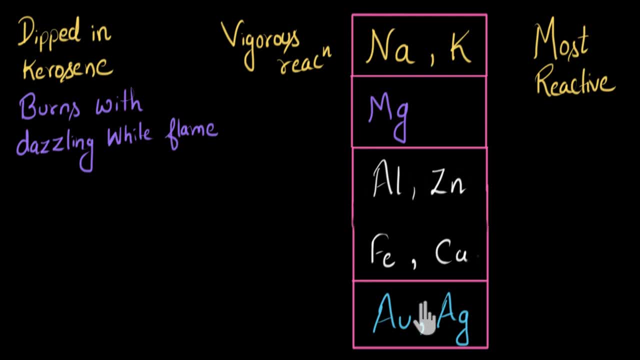 Now these two metals: on being heated up, they do not react with oxygen, Doesn't matter how much so ever you heat them, there will be no reaction happening. That's why these metals are called noble metals or peaceful metals. These are the least reactive in our list. 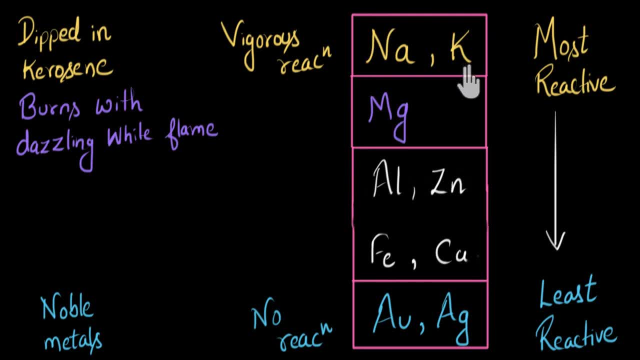 So this is our list of reactivity. Here the metals sodium and potassium are most reactive. Then we have magnesium. Then we have these metals, aluminum, zinc, iron and copper. We are not sure which one is more reactive among them. 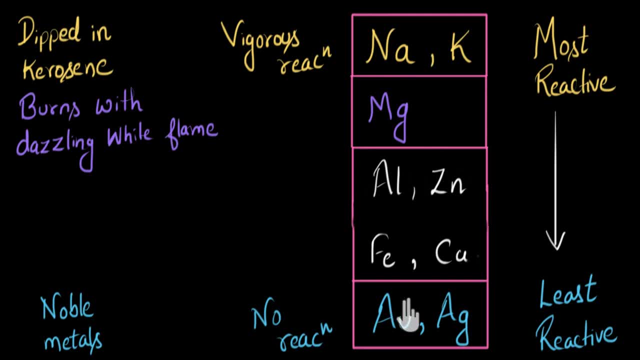 And then, at last, we have gold and silver. Now, before we wrap up the video, let me tell you one interesting fact. See few of these metals. they can react with oxygen And form oxides, even at normal temperature, without being heated up. 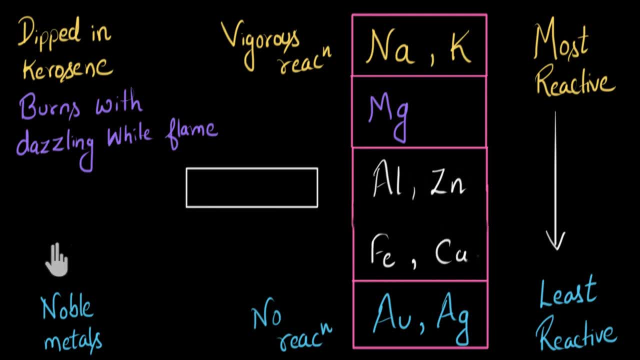 For example, if I take a piece of aluminum metal and I leave it outside for some time, Now the outermost atoms, the ones that are in contact with air. they can react with oxygen and form oxide, even at room temperature, even at normal temperature. 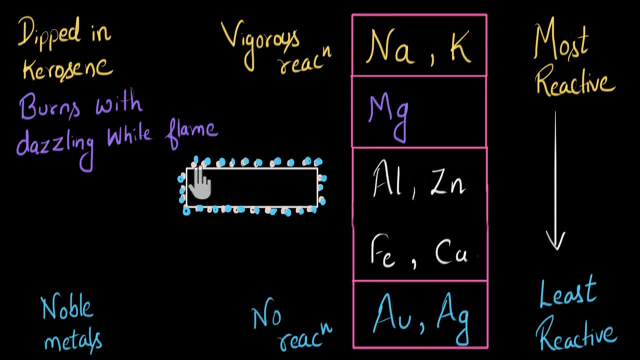 Something like this, And they will form a protective layer, a layer of oxide, Over this metal. So what will happen is this layer will prevent the innermost atoms from reacting with oxygen, Because now oxygen cannot go through it and come in contact with the innermost atoms, right? 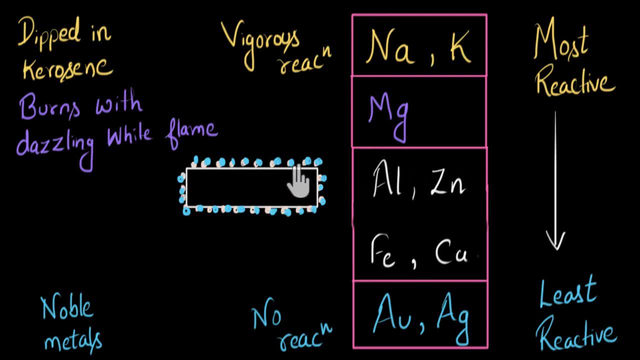 So in one sense we can say that the outermost layer, it sacrifices itself by reacting with oxygen And therefore it prevents or safeguards the innermost atoms from reacting with oxygen. And this happens with With many metals like magnesium, zinc, sodium. they all will have a layer of metal oxide. 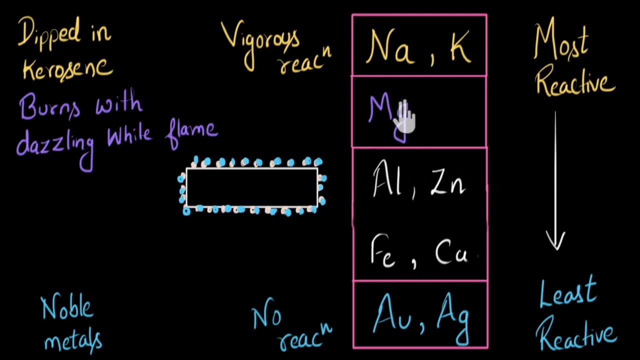 on top of them. In this video, we wanted to rank the metals in the order of their reactivity. For this, we reacted the metals with oxygen and let them form oxides. Now, depending on how vigorous the reaction was, we put them in this particular order.